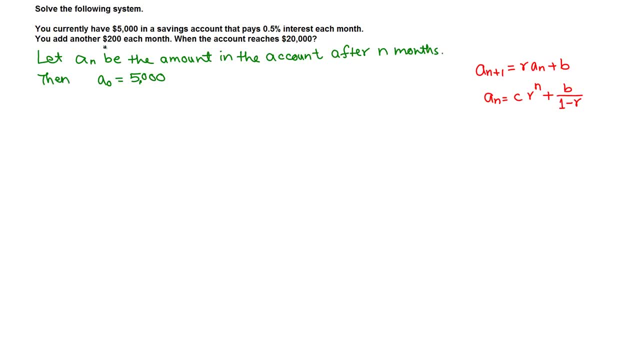 Solve the following system or the following problem. You currently have $5,000 in a savings account that pays 0.5% interest. each month. You add another $200 each month and the question is when the account reaches $20,000.. Okay, so let's assume let A and B be the amount in that account. 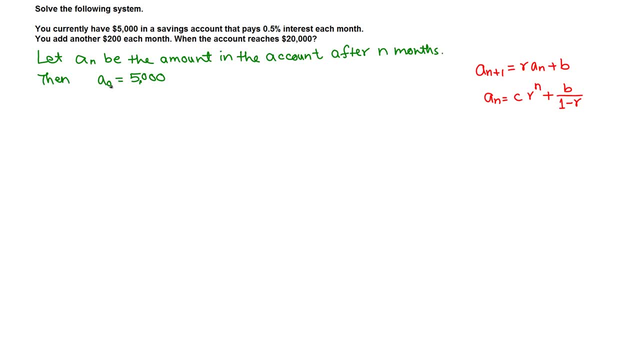 after n months, then after zero month. that means at the beginning A0 is $5,000.. Now the system will be the following: what will be the amount in the next month? So an plus one is equal to the previous amount. in the next month is an plus the interest earned on an. the interest earned on this. 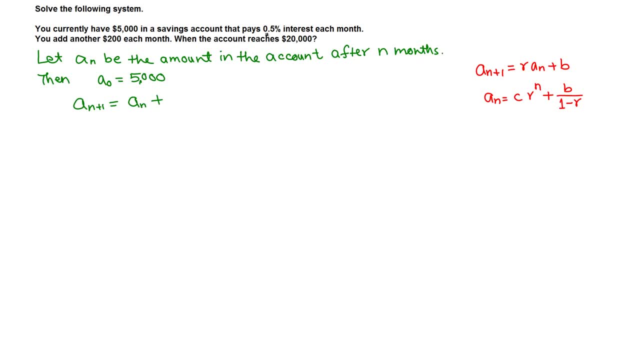 an is 0.5%, need to divide by 100. that gives you 0.005 on AN. that's the interest and we add $200.. Okay, this is the system. that is. AN plus 1 equals we can add these two terms. so one copy of AN, 0.005 AN. so 1.005 copies of AN. 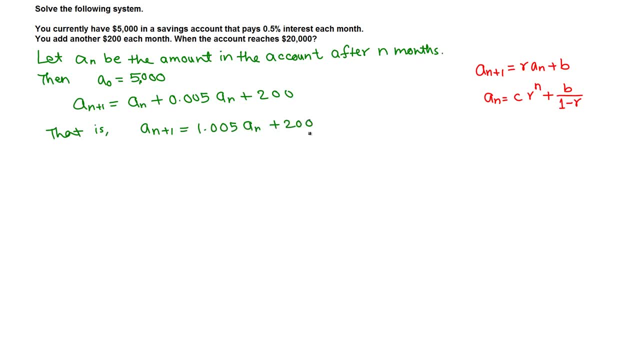 plus 200.. Now this system with A0- 5000 looks like this and this is the solution. the solution is given by C times R, raised to N plus B, over 1 minus R, when R is not equal to 1. otherwise we will be dividing by: 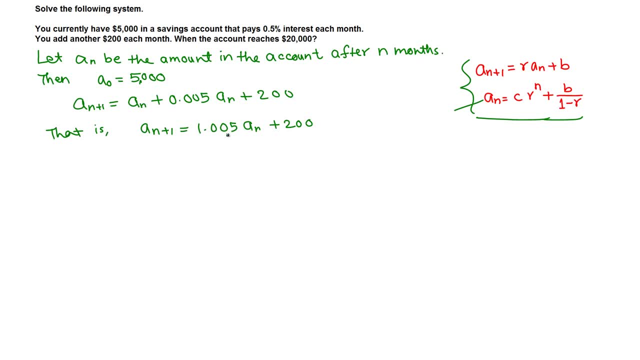 0. that's not the case. R is 1.005.. Okay, now then solution, or all the AN's can be written as follows: AN equals CR, R is 1.005 and CRN plus B. B is 200 over 1. 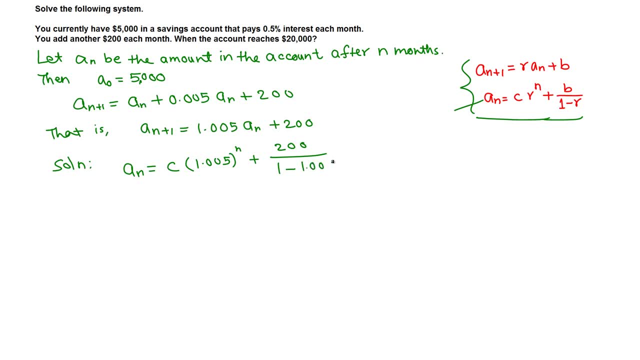 minus R, R is 1.005.. Okay, That's for all. N equals 0,, 1,, 2, 3, etc. That is AN equals C times 1.005. raised to N, 1 minus 1.005 is negative 0.005. now divide 200 by that number and that gives. 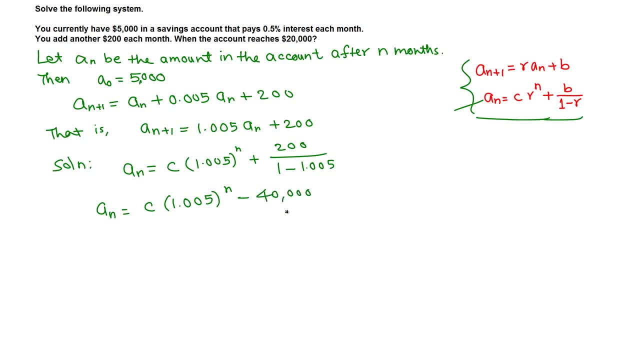 negative 40,000.. Next, to determine the value of C, we use the initial value: A0 equals 5000. so using A0 equals 5000, we get A0, N equals 0, so that's 5000 equals C times 1.005 raised to 0, because A0 means N is. 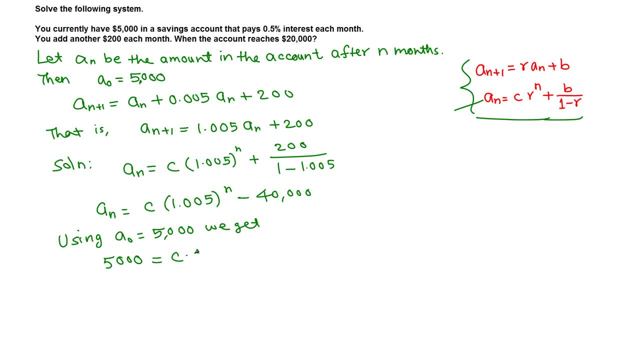 0 and a number raised to 0 is 1, so C times 1 minus 40,000.. So this is C. Now to isolate C, we add 40,000 both sides, then that implies C equals if we add 40,000, so this becomes 45,000.. Okay, thus AN is. now let me go. 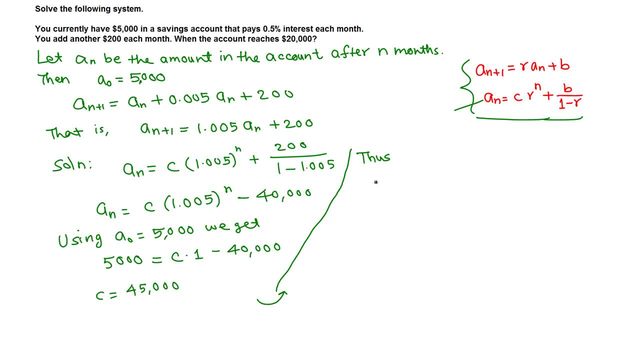 over here. thus AN is equal to: from here C. we just found 45,000.. Okay, so we have C times 1.005 raised to N minus 40,000. for all N equals 0,, 1,, 2,, 3,, 4, etc. 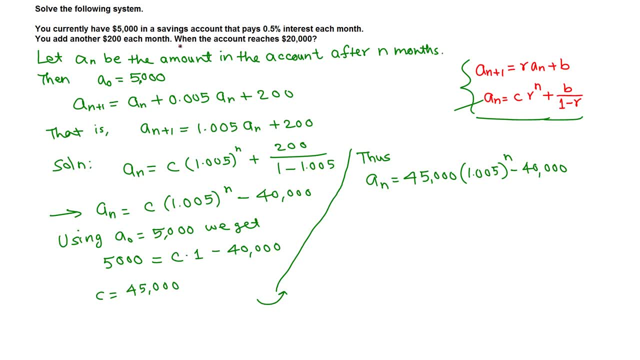 Okay. now the question is when. that means after how many months the account reaches 20,000.. So this is the amount after N months. Okay, so our AN is now 20,000 and we want to find N. Okay, set AN equals 20,000 and solve for N. 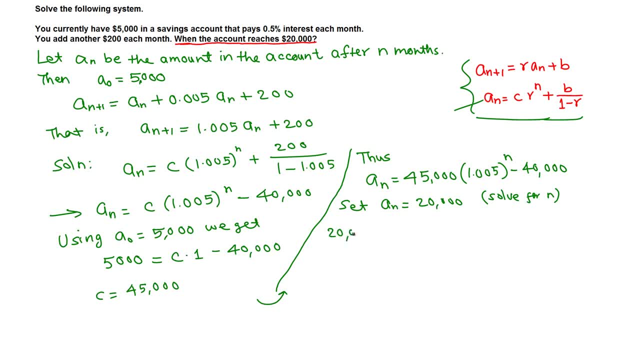 So our AN is 20,000 equals 45,000, so N is unknown. that's what we are trying to find: 1.005 raised to N minus 40,000.. Now 40,000, 20,000. so add 40,000 to both. 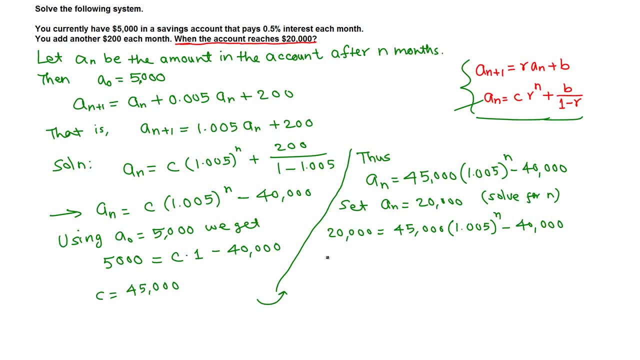 sides moving this over. so when we add 40,000 it becomes 60,000. equals 45,000 times 1.005 raised to e, N. We are trying to solve for N, so move 45,000.. That means it's time. so divide both sides by 45,000. so 60,000 divided by 45,000. 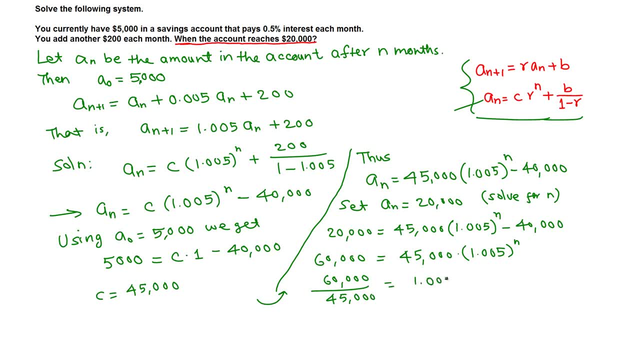 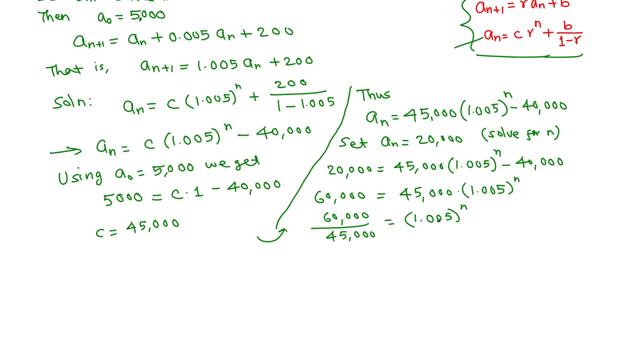 equals 50,000.. 1.005 raised to n. okay, Now we need to solve for n. n is in the exponent, so this is an exponential function. so we have to take natural log both sides. pretty much we can cancel 1000 from top and bottom, 60 over 45 take. 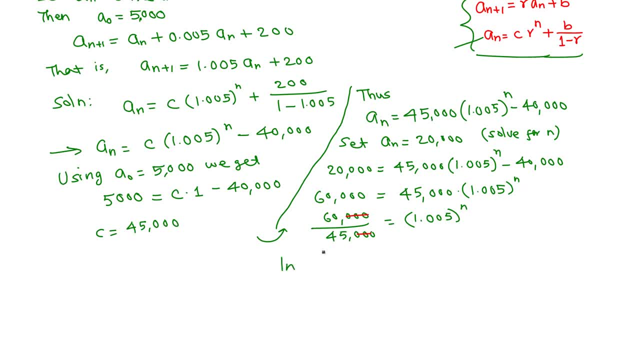 natural log of both sides. we get natural log of 60 over 45 equals. when we take natural log, this n jumps to the ground level, so this becomes n log. natural log ln of 1.005.. Now this is a decimal number. divide both sides by this ln to. 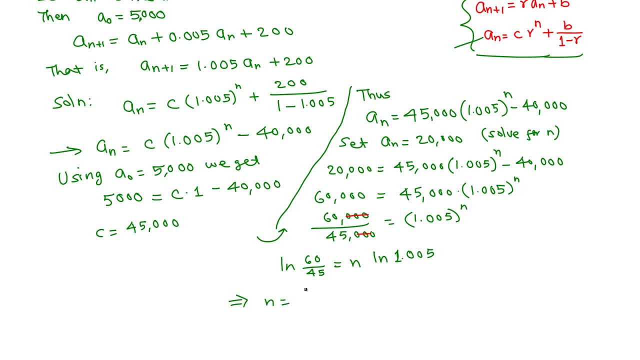 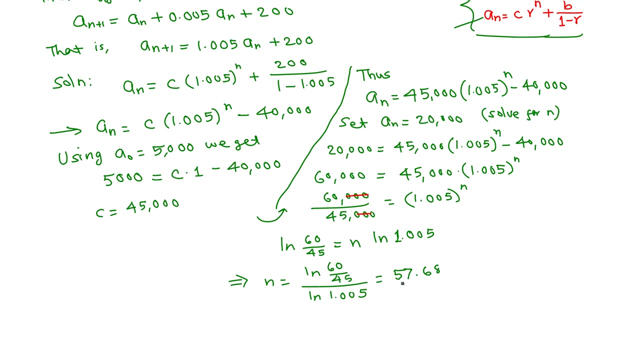 isolate n, So n equals this number: ln 1.005.. 60 over 45 divided by this ln 1.005, now use your calculator- it comes out to be 57.68. that means the account reaches 20,000 after 57 months. and